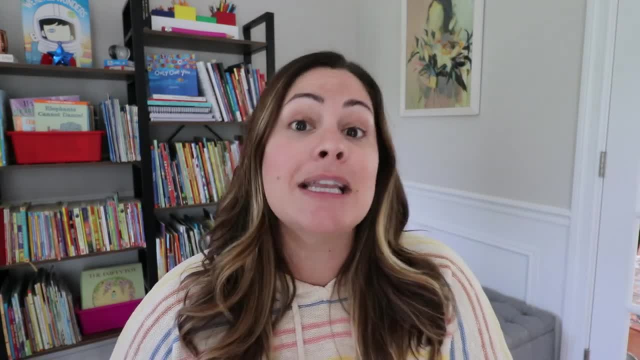 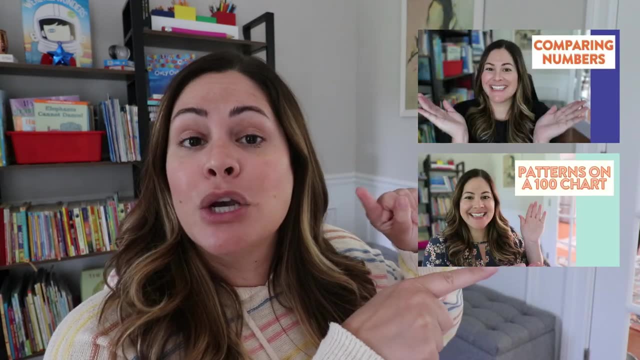 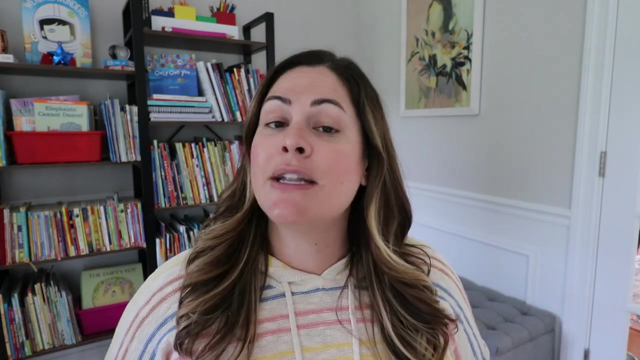 deeper conceptual understanding, as well as some concrete activities that you can take and use with your students right away. So the first video I did was about comparing numbers. last week's video was all about understanding patterns on a 120 chart, and today we're talking place value. Just like in my other videos, I'm 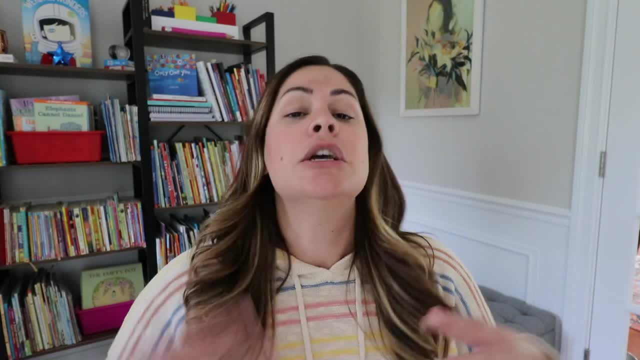 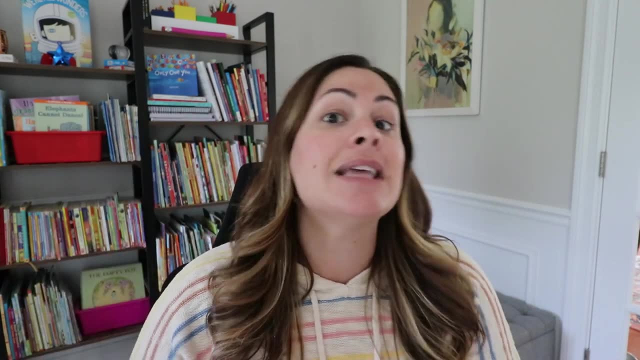 going to give you an example of a lesson you can do with your students to help them conceptualize this tricky idea, and then I'm going to share three fun, concrete activities that you can do with your students to help them with place value. If you're ready to see these ideas, give this video a like. subscribe to my. 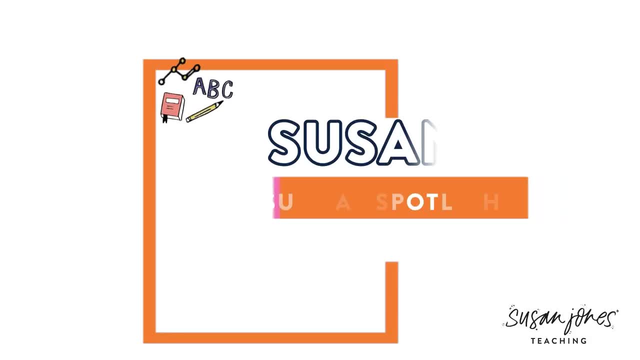 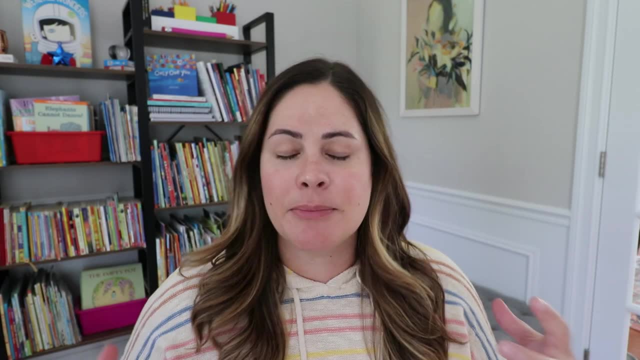 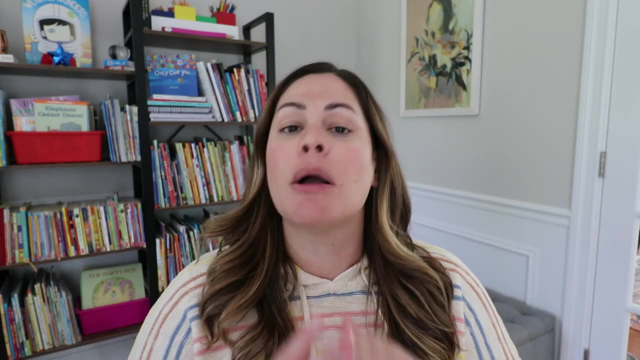 channel and let's just dive in Alright. teaching students about beginning place value, about tens and ones, is the beginning of teaching students how to unitize, and unitizing is probably the most important thing students are going to have to understand in K-2. 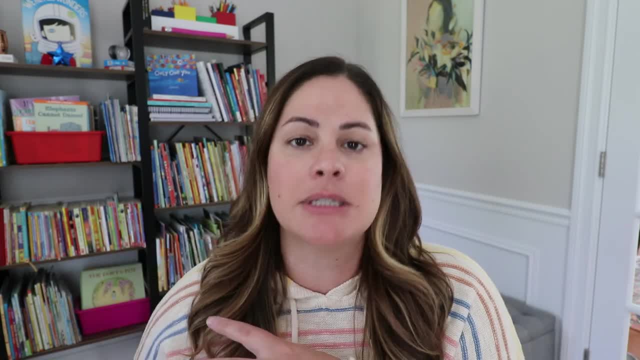 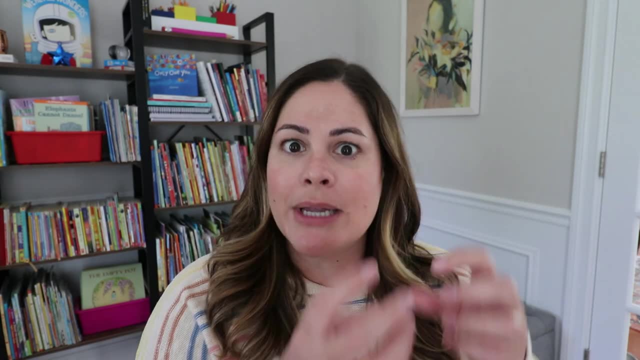 before they kind of build on to more difficult skills right, Especially in K-1. we really want them to understand what unitizing is, and unitizing is essentially grouping things to count them in a more efficient manner. if we're talking about math and with our 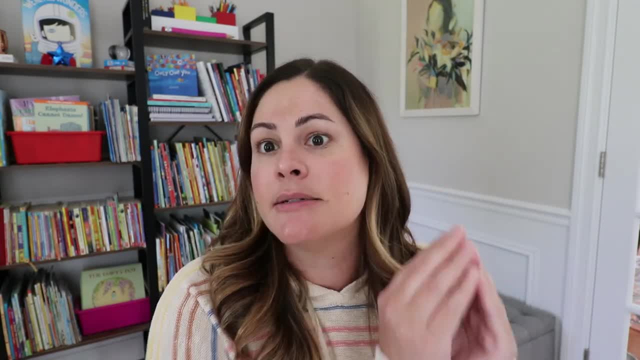 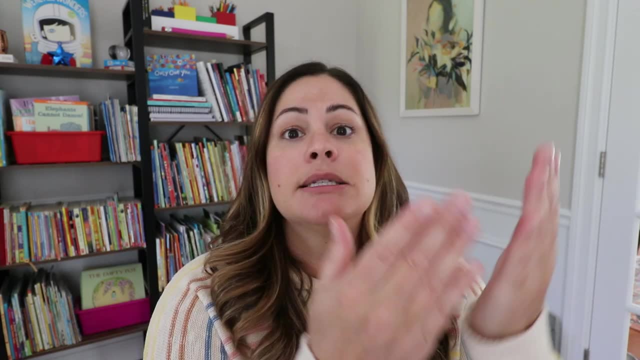 base ten system. it means we're grouping things into tens. As students learn more about the base ten system, they'll realize that not only do we group 10 ones to make a 10, we group 10 tens to make a hundred, 10 hundreds to make a thousand. 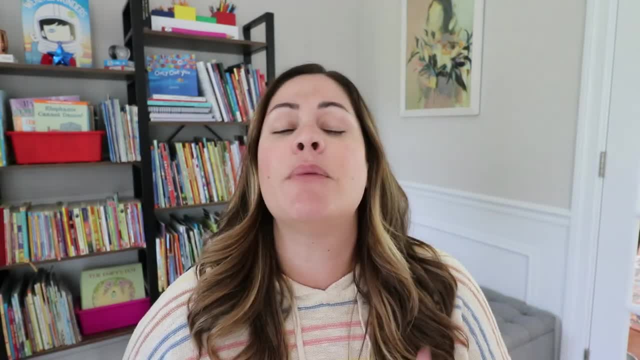 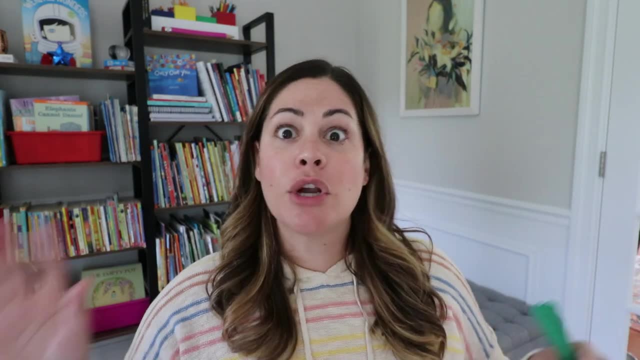 and so on, But our goal as primary teachers is really to help them understand and get used to that idea of unitizing so that they can do it efficiently. Alright, before I go into this lesson, before you would start this lesson with your students, 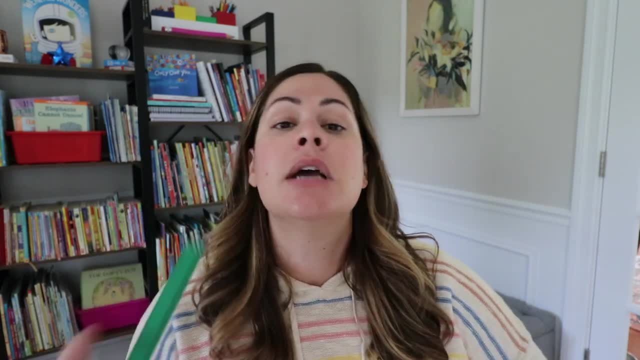 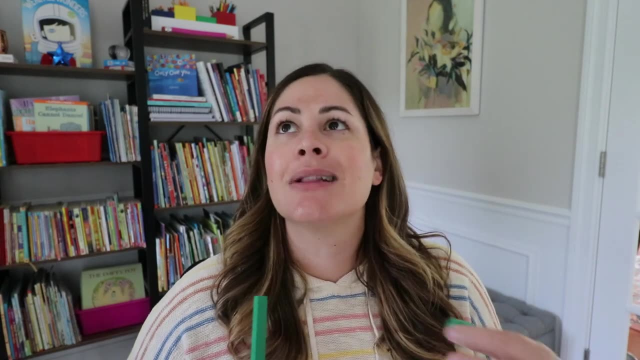 your students should have some knowledge about base 10 blocks or if you're using unifix cubes, that's fine, but they should know how to represent a number using tens and ones, or at least have done it. you know a couple times, have seen you do it. they should understand that this is a 10. these 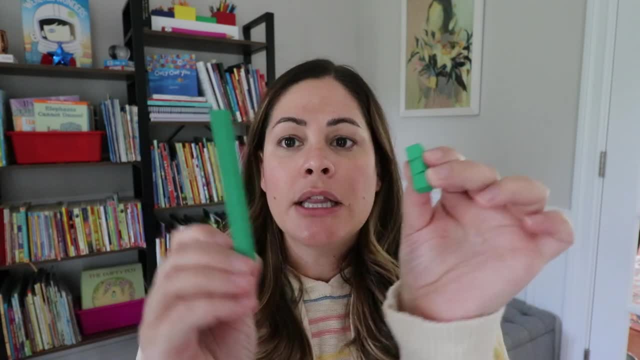 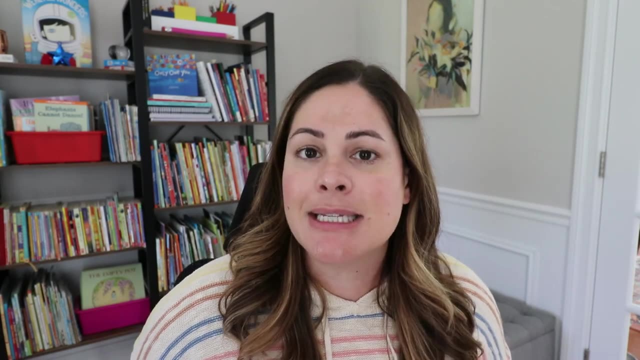 are some ones, and i don't know how well you can see this, but this number together would represent one, ten, three ones or thirteen. now, when having students do this conceptual lesson, i would have them work with pairs and in their pairs they're going to need some base 10 blocks. they're going 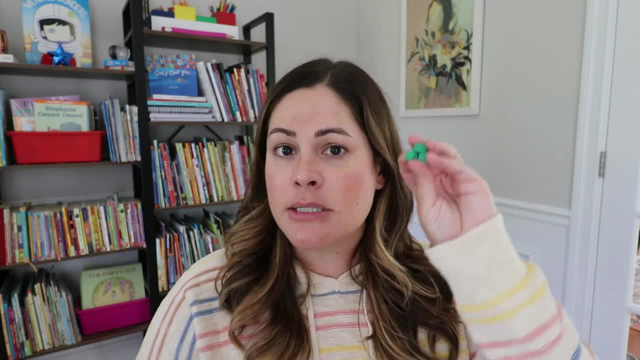 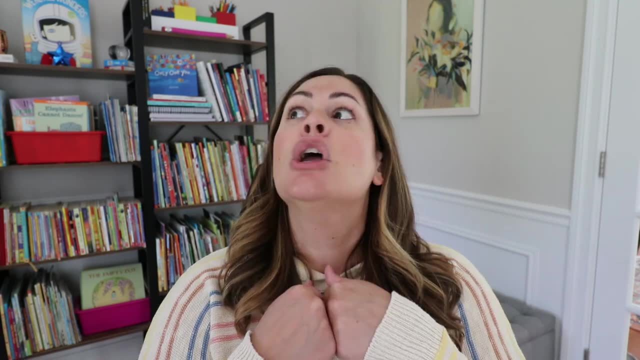 to need some rods here, some tens. they're going to need a bunch of ones because they're going to show numbers in different ways. once students are partnered up and they have their materials, i would pose to the class. i would say, using your base, ten blocks with your partner, can you come up with a? 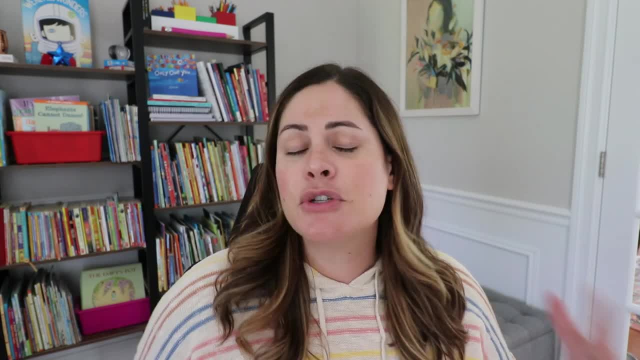 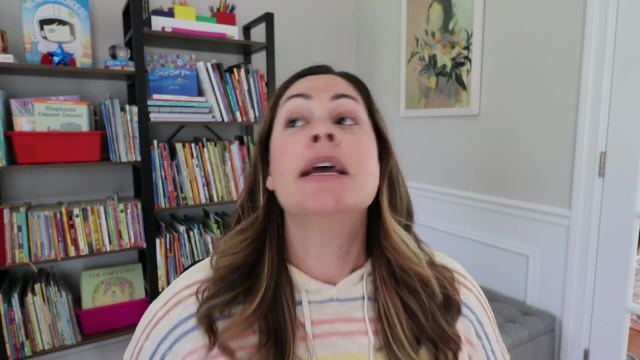 way to show the number 26. give your students about a minute to figure this out and most of them are going to show you two tens and six ones with their base ten blocks. Now, if you have some other students that are like, ooh, I'm going to do it a different way, 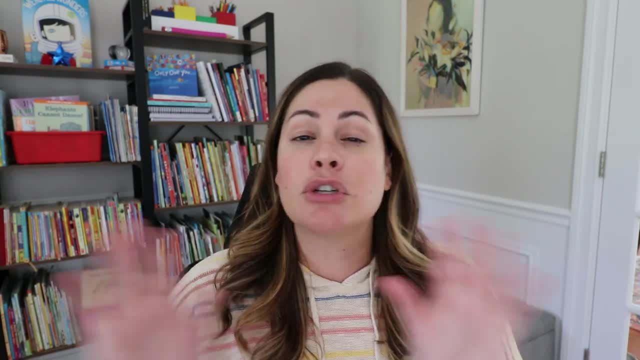 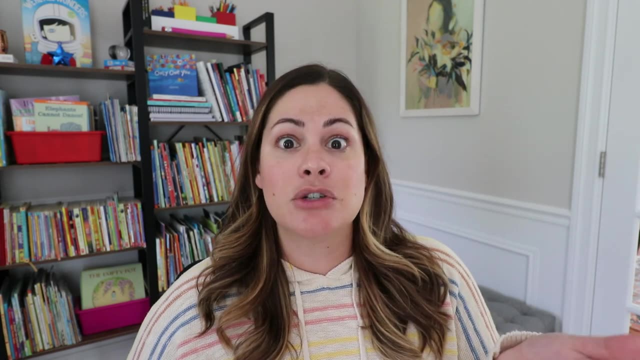 maybe they will have shown you 26 ones. Those are usually the two first ways, if they do a second way at all that your students will usually show And, of course, ask your students to come up, maybe show it under the doc cam or draw what it looks like on the board. 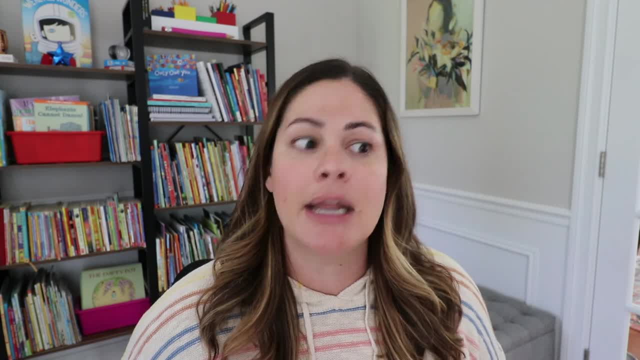 explain it to the class and have other students repeat what they said. How did so-and-so go ahead and build it? Is that different from what you had, or is it the same? Do you agree, Do you disagree, And so on. 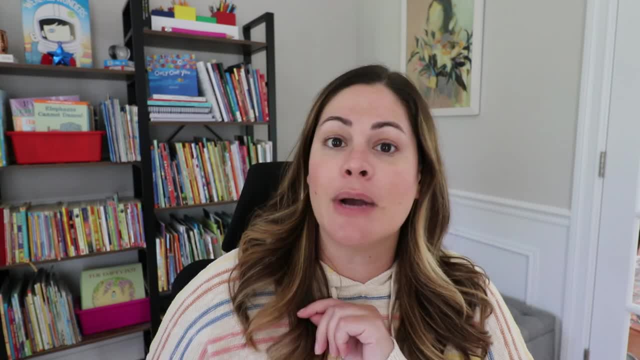 If you do have a pair of students that does it in a different way, be sure to highlight that. ask the class if anybody did it differently. And even if they didn't, that's your next step. You're going to say: is there another way? 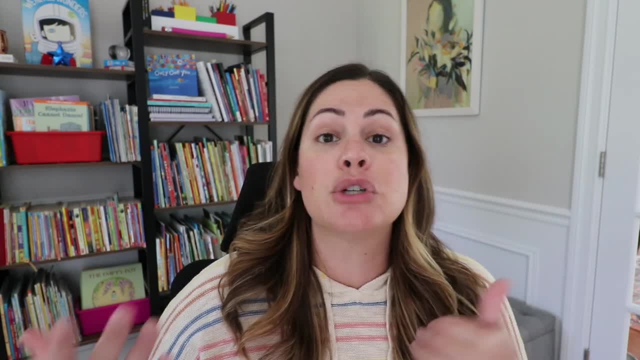 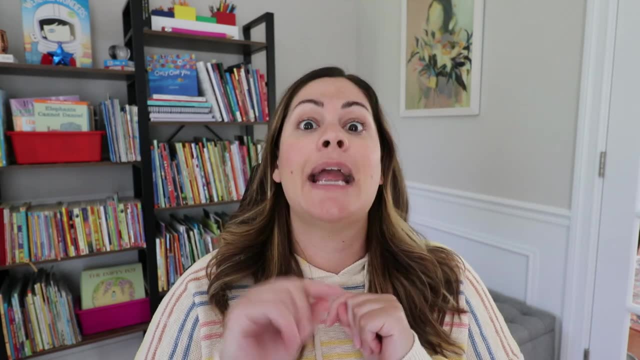 using your base 10 blocks in front of you, that we could show the number 26 and see what they say. Usually, the last way they find is that one where you have one rod and 16 ones. So here would be the three ways that your students could represent. 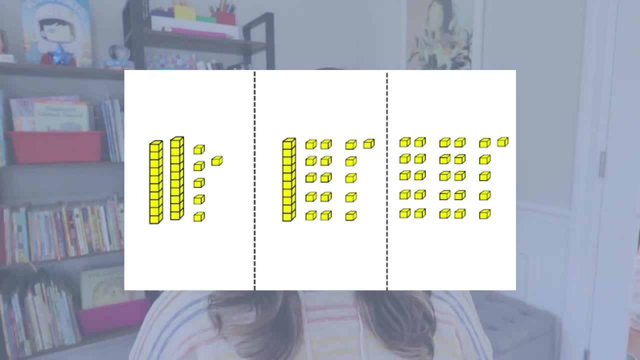 the number 26 using base 10 blocks. Once you guide your students to getting these three ways, we have some questions I want to ask about these numbers. So first we'll take a look at all three representations And I would ask the class: are these numbers equivalent? 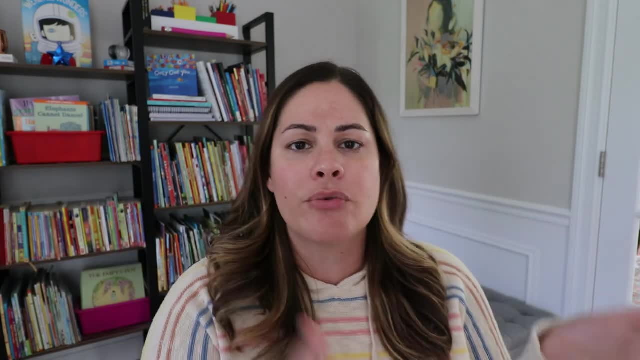 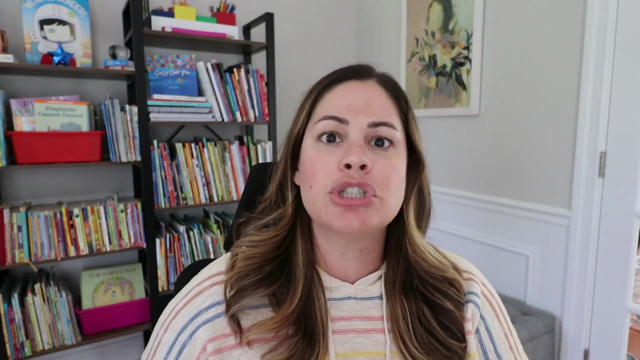 Are they equal? And students will have to figure out if all three of these representations are equal. How are they going to do that? Have them explain it to you. How can they prove or show that you know two, 10s and six ones? 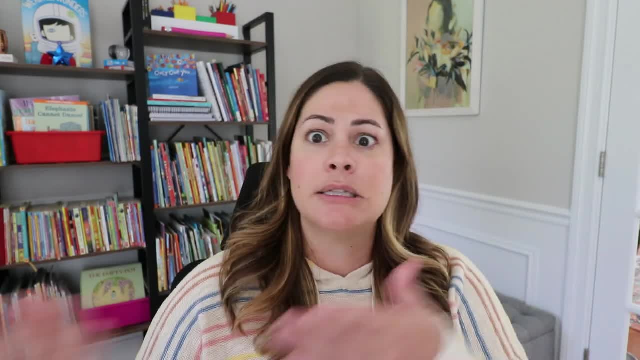 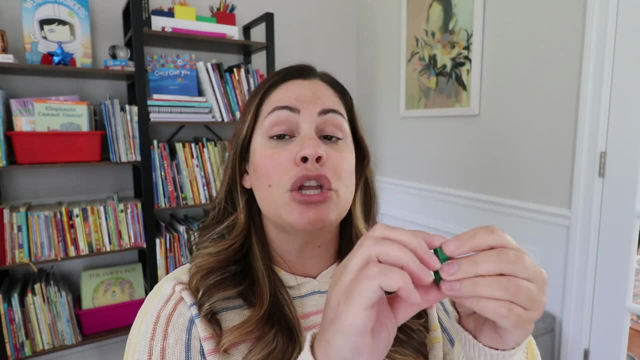 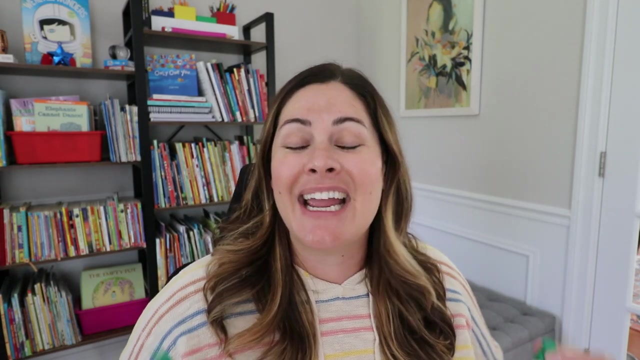 is the same as one 10 and 16 ones, And are both those the same as just 26?? How can they prove it? Your students will likely figure out that they can go ahead and unitize those ones to represent. They can show how a 10s rod really equals 10 of these ones here, that they are the same. 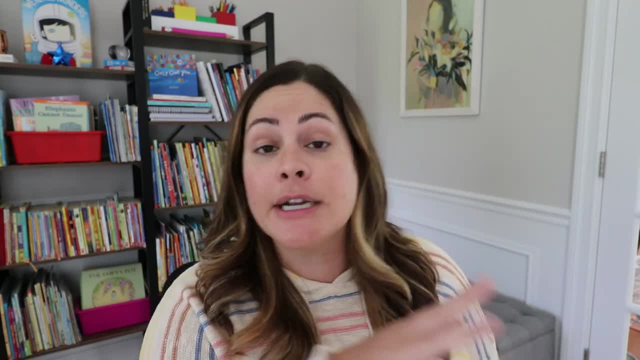 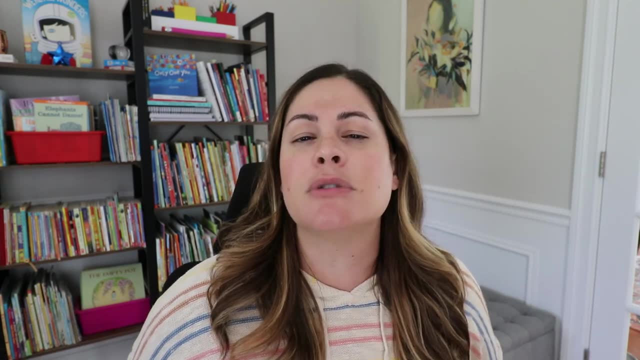 Of course, just a reminder, be sure to ask a few different students: agree, disagree, tell me more, restate what they said again, using all those math talk stems that we know about to really help students understand this even further. 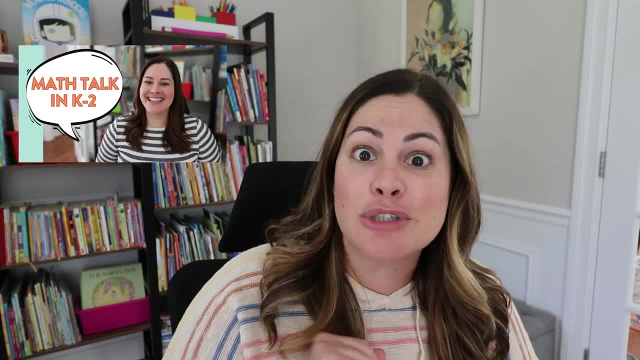 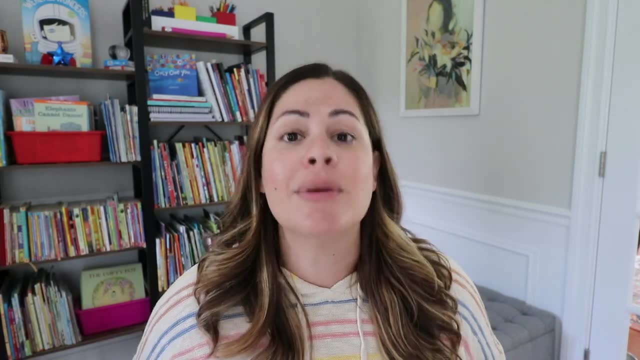 And, as a quick reminder, if you're looking for more of that math talk, that's the video to go check out. Make sure you have all three ways you can make the number 26 on display, whether you drew them on the board or they're under a dot cam. 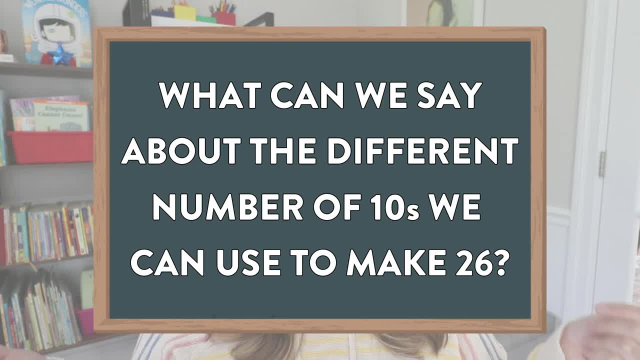 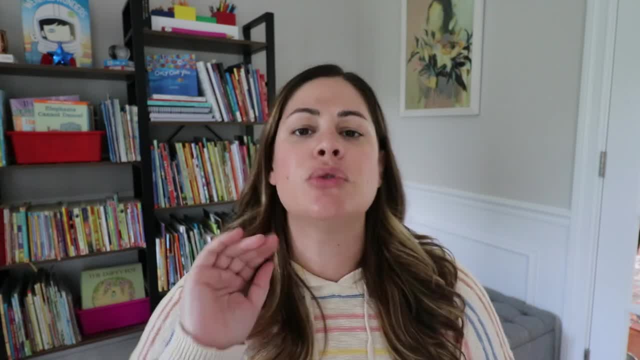 and then ask them: what can we say about the different number of 10s we can use to make 26?? And then hopefully you'll get some interesting conversations. They'll realize that there's two, there's one, there's zero. 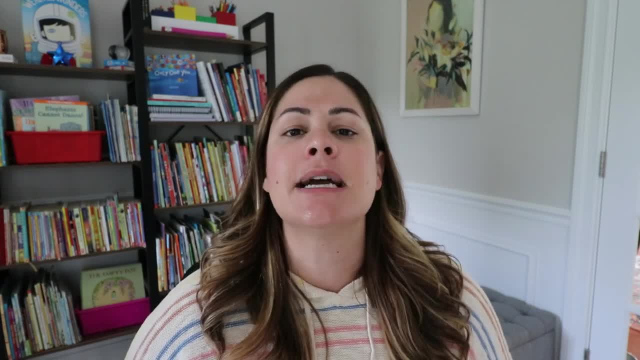 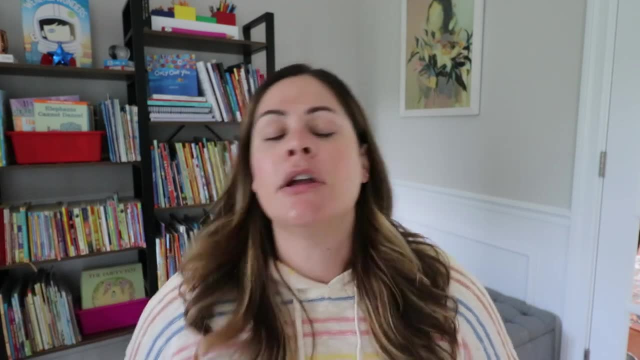 but they all equal the same thing. But then you can go on further and ask them: well, what if I take those 26 ones, and how could they make them look like the other ones? What could I do? You know, they would say, you can group the tens. 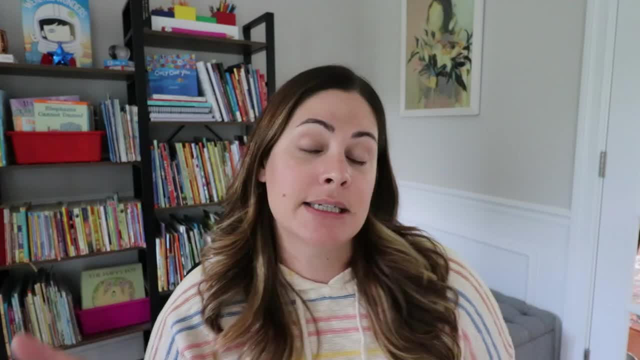 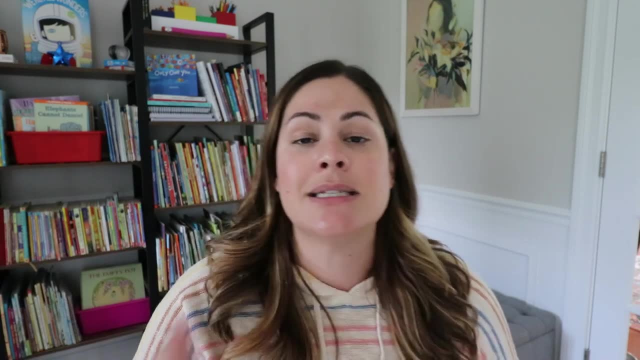 make one ten to make it look like the second option, where there's one ten and 16 ones, or you can continue regrouping, right, You can make another group of ten to make it look like two tens and six ones. I talked about this before, but the importance of conceptualizing 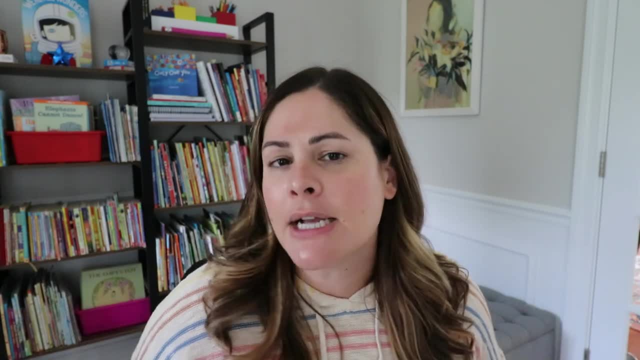 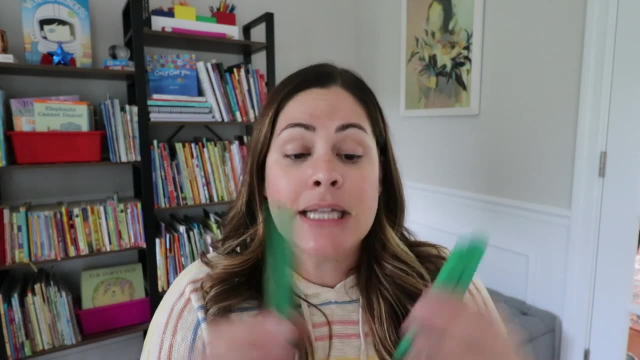 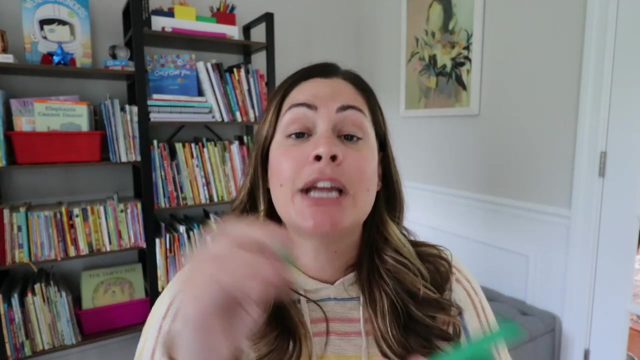 these skills is so that students are flexible with their thinking and they're flexible with numbers. This helps students really understand and see multiple ways and hear multiple different ways, that tens, a tens rod, is the same as ten singles, ten units. They're the same thing and they can be interchanged and exchanged. 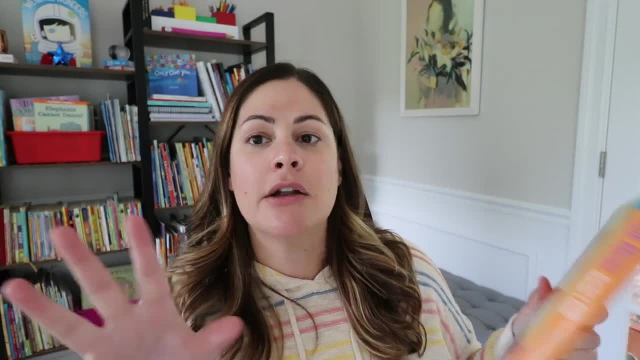 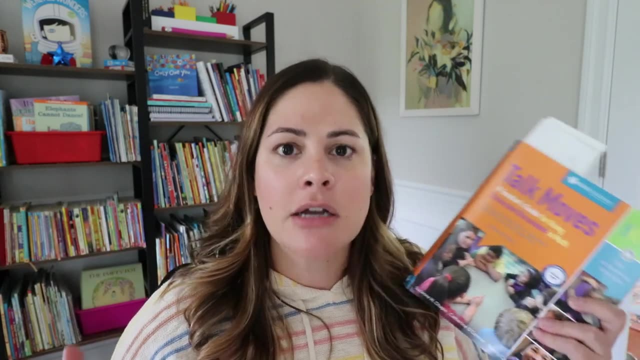 to show different options of making the same number. Now I want to share. I got a version of this lesson from this book right here. It's called Talk Moves. I love this book for promoting mathematical talk and mathematical concepts in your classroom, And the teacher in here is a first grade teacher. 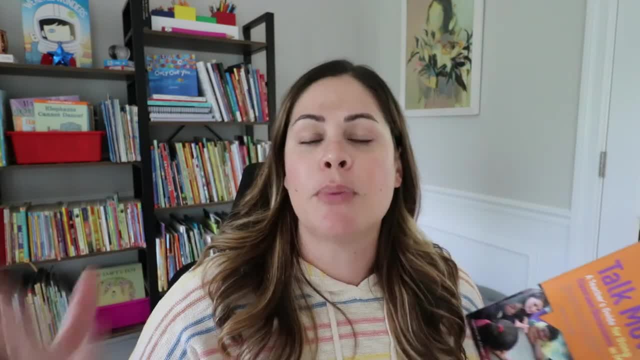 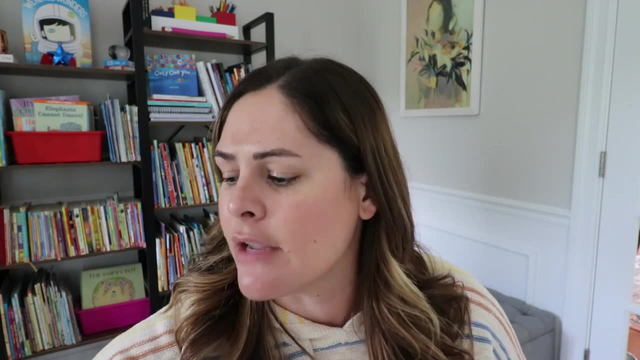 that did a very similar lesson to this one when she was proposing this to her class, especially this last part about using the tens. One of her lessons was about using the tens. One of her students asked they were like: well, wait a sec if I have one, ten and sixteen ones. 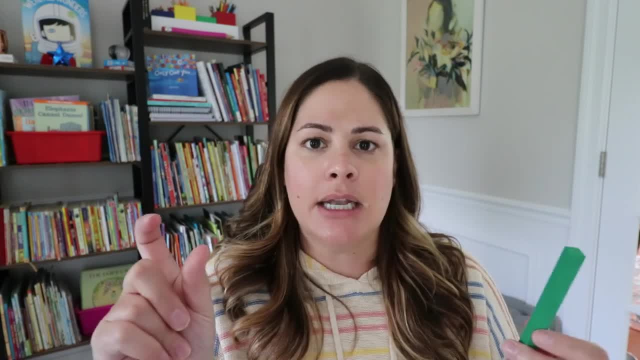 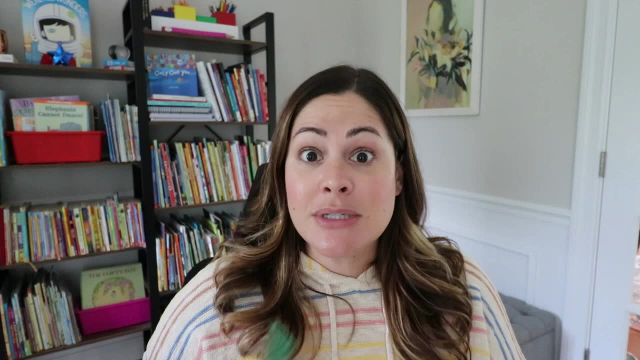 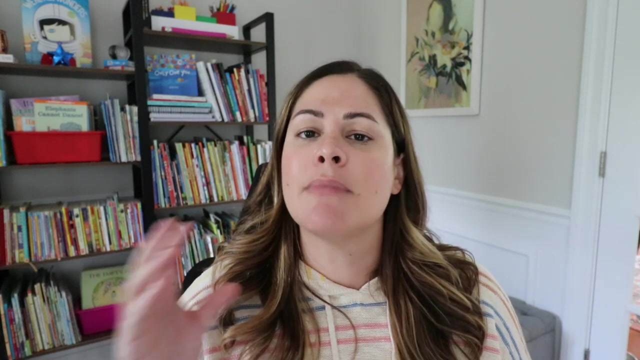 how can I write that? I can't write one sixteen because that would look like one hundred sixteen instead of twenty six. And one of the amazing things about using consistent math talk in your class and having students ask questions and talk about math a lot is that you can see where there might be some misconceptions, some confusion. 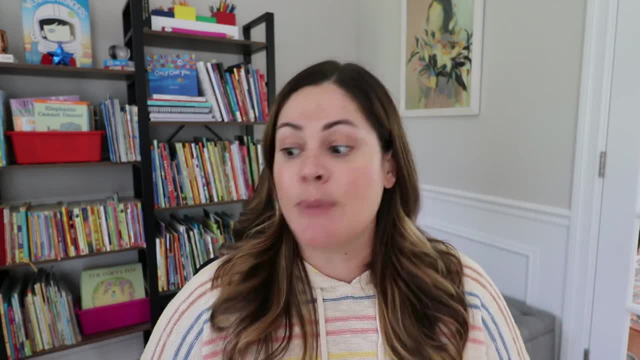 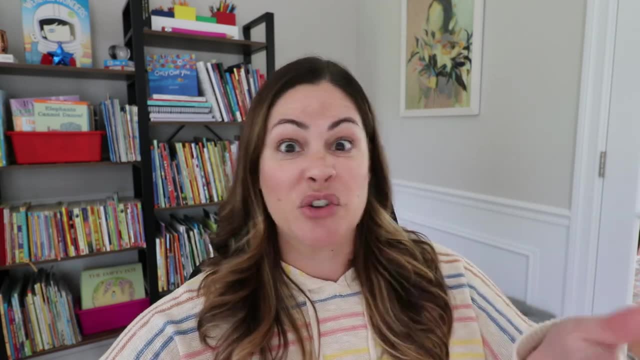 And for the teacher, this was a great eye opening kind of moment. She wasn't expecting this. She wasn't expecting this question about how do we actually represent it when writing. So it was a great time for her to take this opportunity and say: you know what? you're right. 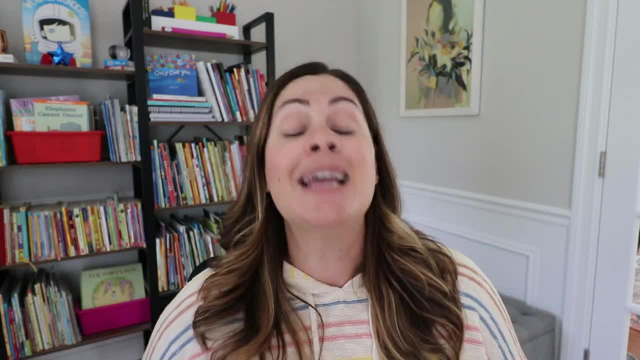 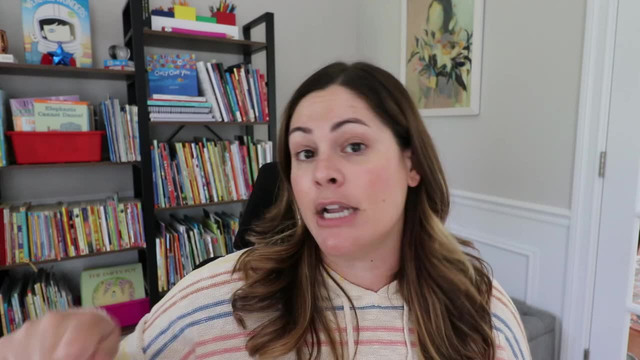 If we write one one six, that's one hundred and sixteen, And that's why it's so important that we unitize whenever we can, especially when representing and writing our numbers. We need to go ahead and group as many tens and then, as they get older, 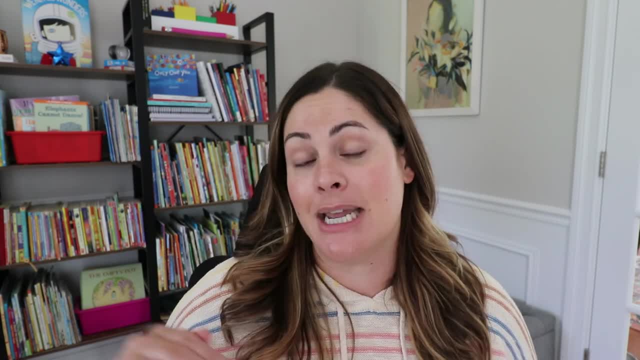 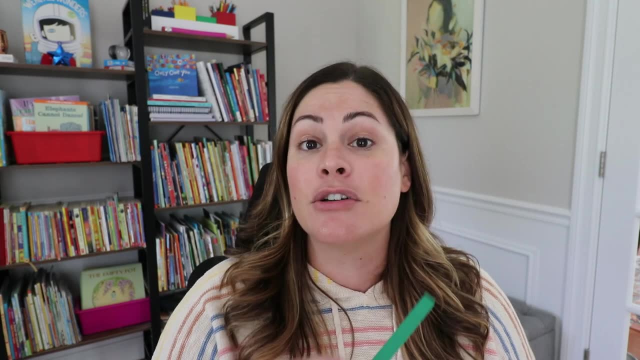 hundreds, thousands as we can to write it down in our base ten system. So in our system we have to show the maximum number of tens. You can make that two for twenty and then all the leftovers, the six, After reading that in the book. if I were to do that lesson with my class, 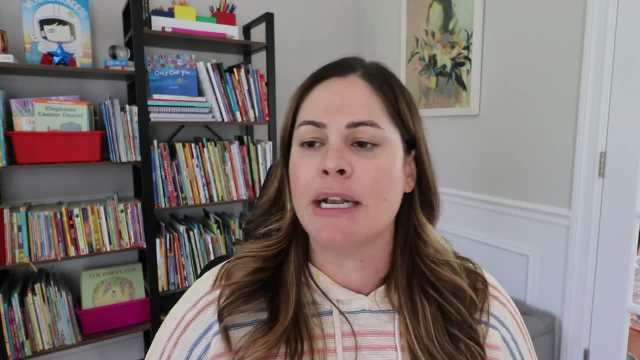 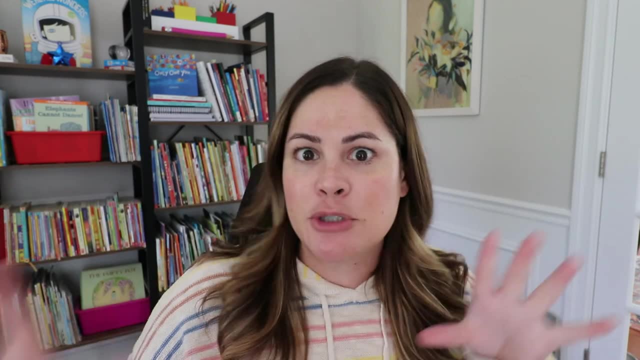 the way I explained it to you. I might even bring that up later. I might even ask them: well, hey, wait a sec, how could I write this? Just to make sure that they understand this too. All right, So that's an example of a great conceptual lesson to get your students. 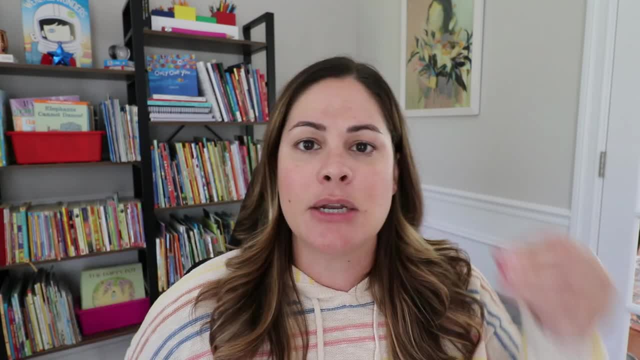 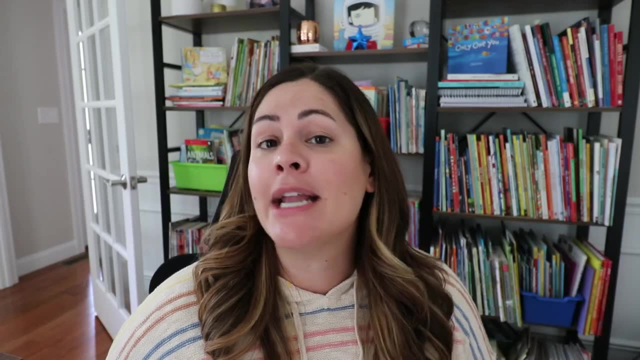 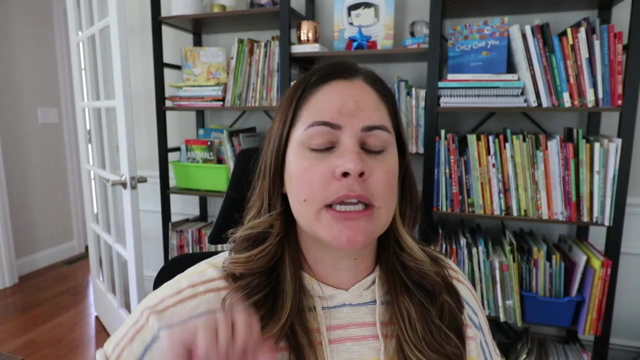 talking about number sense, place value, tens and ones. So now let's go over some concrete activities you can use with your students. I have shared quite a few place value activities. that are some of my favorite, But when specifically thinking about tens and ones, I narrowed it down to three of my faves. 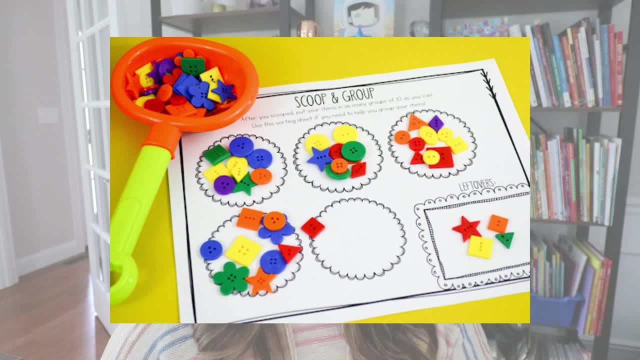 First is the activity scoop and group. Now this activity is such a great one for students to practice unitizing and really grouping items into tens. Now for this you can use a bunch of different manipulatives. in this picture I used all these little shape buttons here. 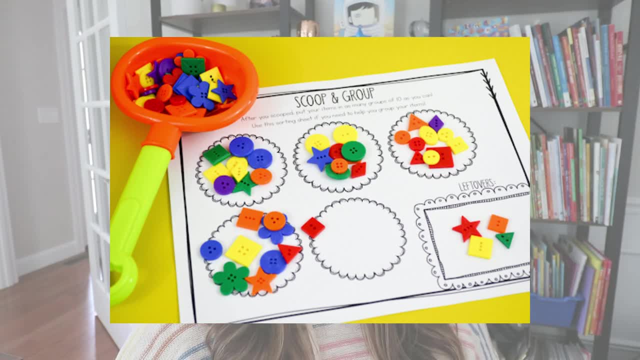 I even put them in a little summer pail with a little shovel and I would have students close their eyes. They would reach in. They could either use the shovel or they can just use their hand and take a big handful. Once they do that, they need to actually count those items into groups of ten to place them. 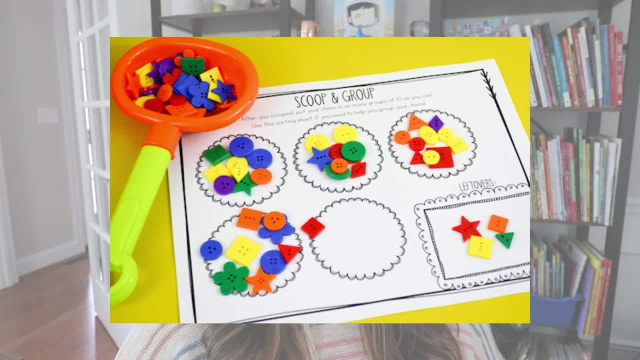 in the circles. So once they've done that, they get an entire group, And every time they get a full ten it will go in one of those circles And then there are some leftovers. Now, in this picture I was a little sloppy. 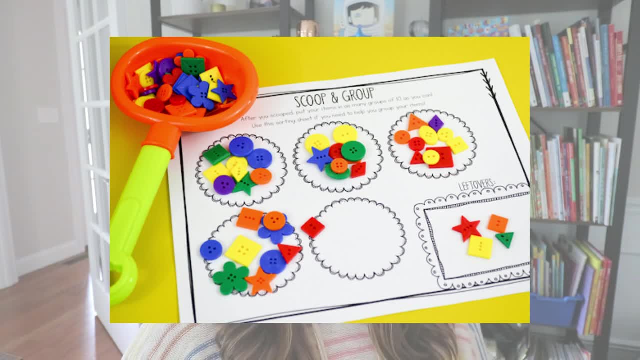 You can see down here that little red square. It should be in the group on the left, But here we have four tens. So they would count up ten, Twenty, thirty, forty And four leftovers to get a number of forty-four. 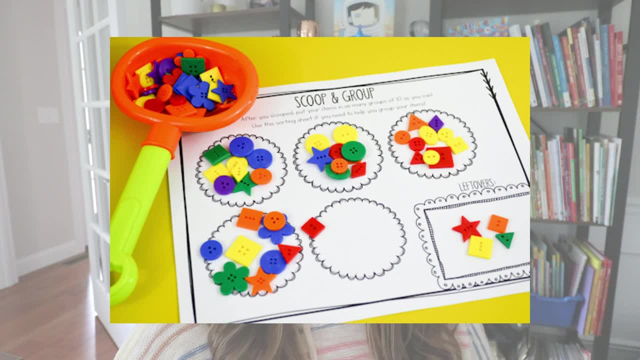 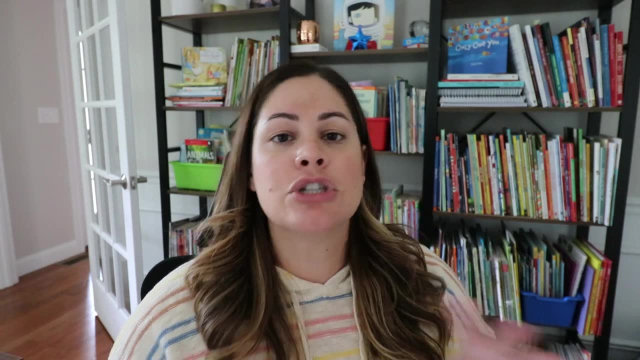 Then students can put all the buttons back in the pail. They can go ahead and scoop another amount and group them. That's also a great one to play over and over again by switching up the manipulative. If you make it larger, the numbers will be a little smaller. 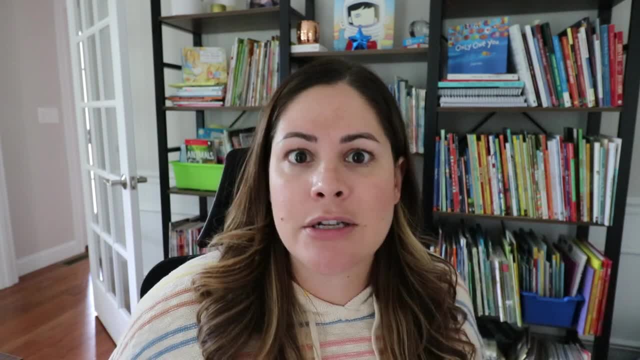 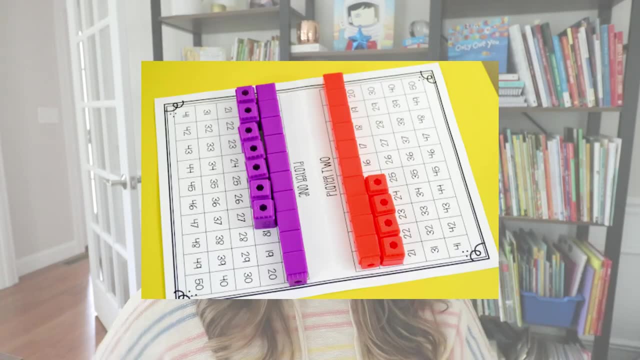 If the manipulative is even smaller, the numbers could get bigger, So on and so forth. The next game I love that really emphasizes tens and ones in the concept of unitizing is Race 250.. Now, this game has been around forever. There's Race 250 or Race 200. 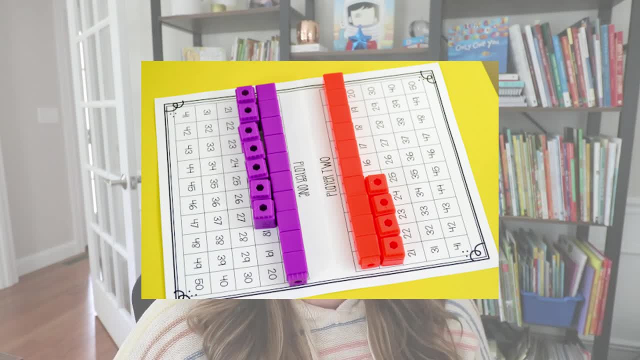 And I like to use this game with Unifix cubes like I've shown here. This is the Race 250 version. There's a player one and a player two, And all students will do is go ahead and take turns rolling a die. Once they roll a number, they will have to get that many cubes. 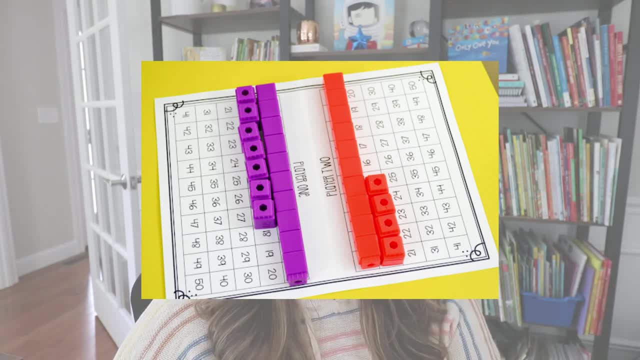 And you can see here how the ones that are still ones- they haven't formed a group of ten yet- are face up And I kind of put them on the little mat there just to show what number we're showing. But then once they're face up, they're not face up. 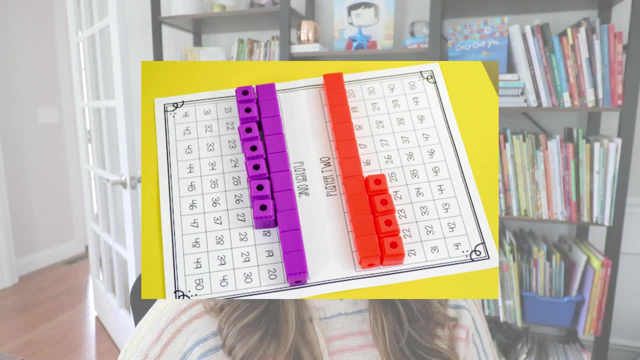 Once students get ten, so as they're adding to their pile, once they get ten, they form it into a rod by connecting all the cubes and laying it down sideways. So then, if I walk over to the groups while they're playing this and I ask them what? 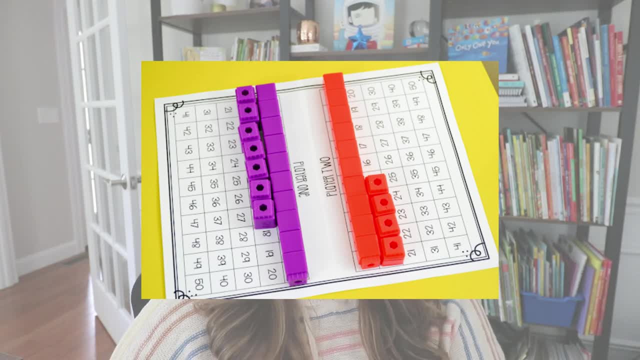 number they have there. I would expect for them to, if I was orange, for them to say ten, eleven, twelve, thirteen, fourteen. Not for them to count up that group of ten anymore, but I'm hoping that they will notice. 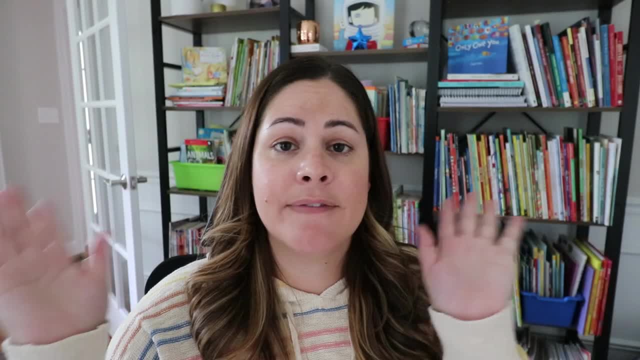 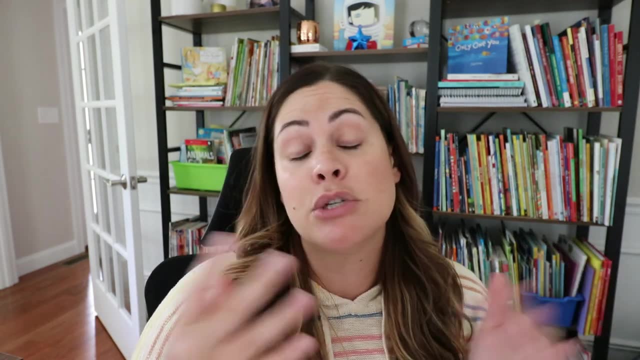 that that is just a ten and that we can add on. And, like I said, I have that exact game. We always start with race to fifty, so students understand how it's played, but then we also have race to one hundred and race to one hundred and twenty for them to play in the same way. 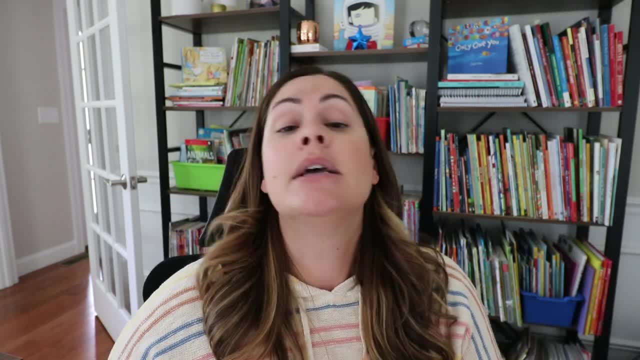 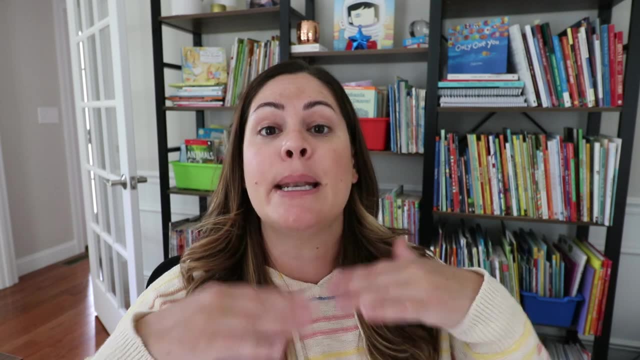 And usually especially for one hundred and twenty. I'll have them use two dice, so they can roll a little faster and they practice a little addition in there too. And last but not least, another easy activity is one you can do whole group and then move. 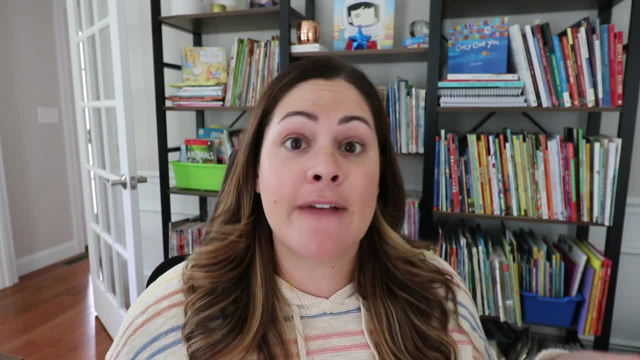 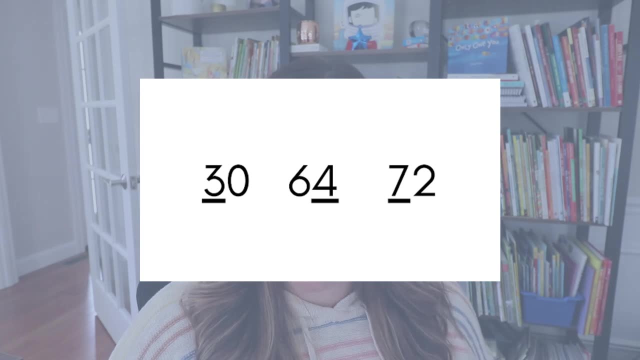 it into some partner games and that is called What's My Value. And for What's My Value, you're just going to show students images that look like this: This is a very simple one. it's not going to be as hands-on as the others, but I like. 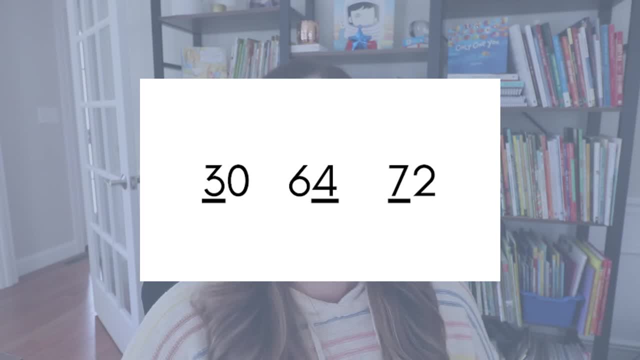 it because it really helps students identify the value of the number in two digit numbers. So here you'll see some examples. I have the number thirty, the number sixty-four and the number seventy-two and you'll see that one of the digits is underlined. 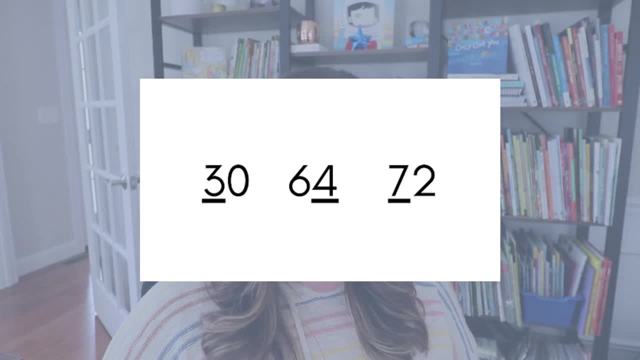 So I ask my students when I'm showing these on the board. I'll ask them what is the value of the underlined number? Because in thirty the underlined digit is three And I'm looking for them to tell me that that means three tens or thirty. 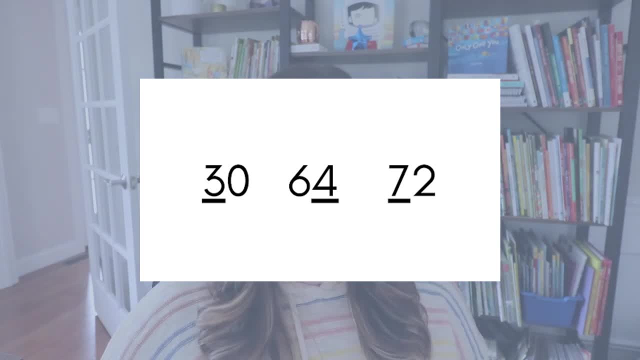 In sixty-four. I'm asking for the value. I want them to tell me that that value is four And a lot of times I'll actually have them represent this. so if we're doing this whole group, I will give them some base ten blocks and they have to show me the value. 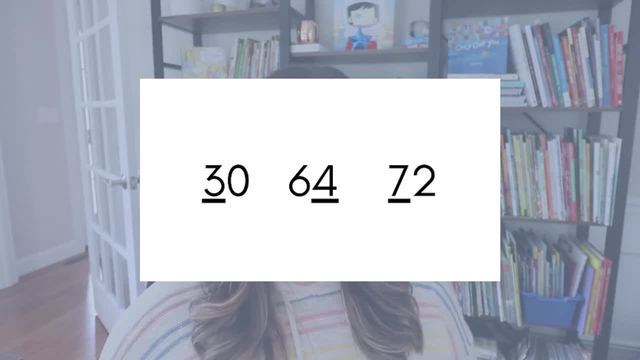 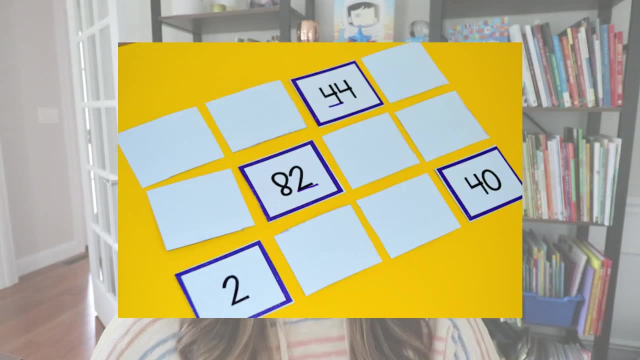 Or if they're doing on whiteboards, they can draw the value and hold it up so I can check When moving this into a more independent or partner game, just to have students reinforce this practice. This is called what's my value memory, where essentially they're just playing memory in. 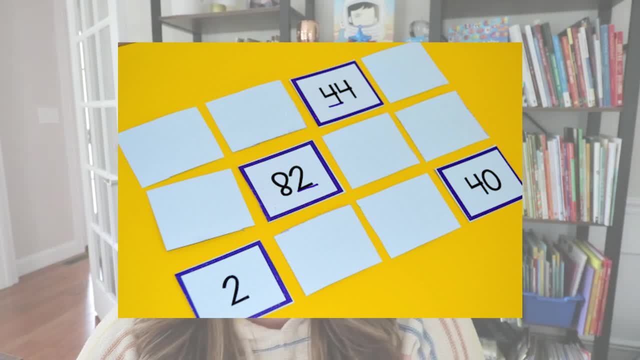 the same way that I just showed you. So here we have forty-four, and the underlined digit is the four, the first one in the tens place. So in order for them to find their match, they have to find the value of that underlined. 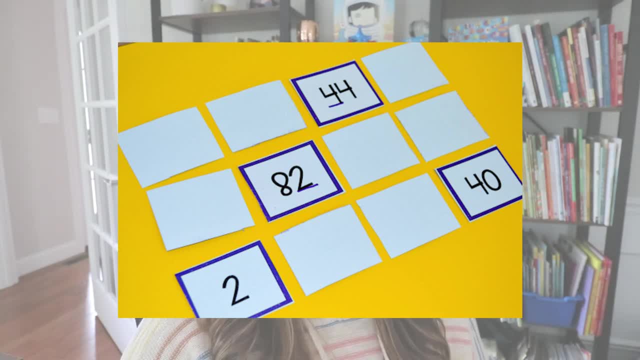 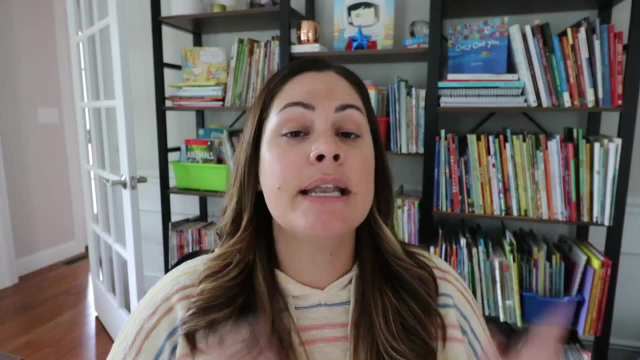 digit, which would be forty down in the bottom corner, Same with eighty-two. the underlined digit here is that two. They need to know that the value of that is actually two ones or the two there. Now the what's the value? memory cards and actually the other two. 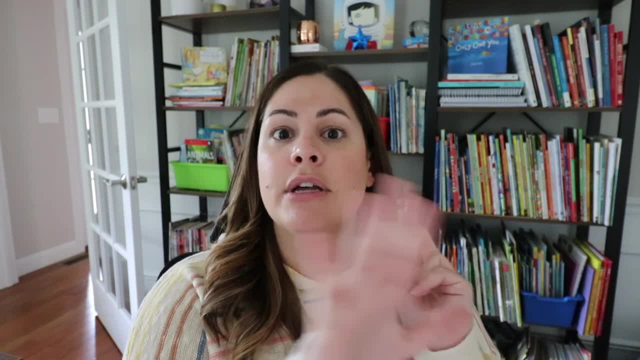 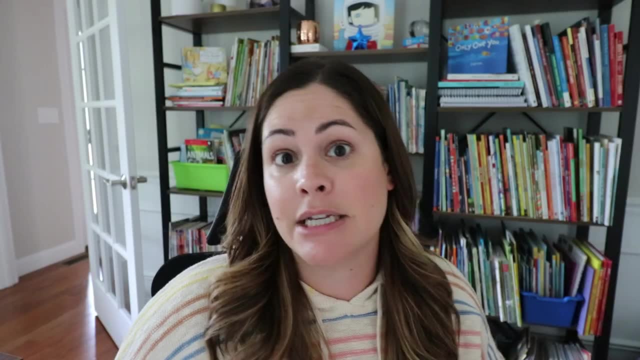 They're all in my activities as well. race to fifty and scoop and group all the sheets that I showed. they're all in my place value unit right here over on TPT. I will link it down below in the description in case you want to check it out. 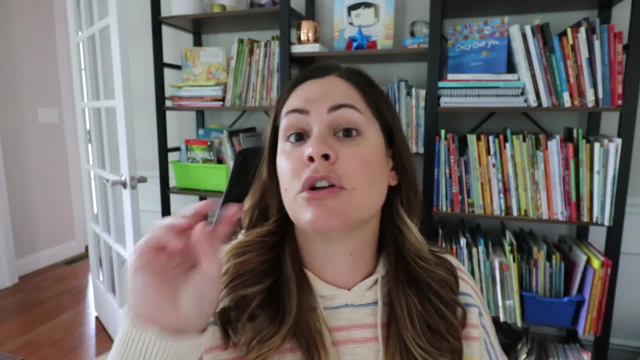 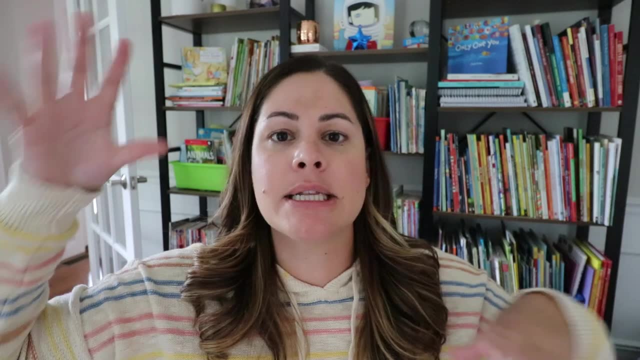 But just so you know, the what's, the value cards, the memory cards. there's also a three digit version as well, so students can understand the value of the hundreds place too when they're ready. So there you have an entire conceptual lesson for teaching students about tens and ones. 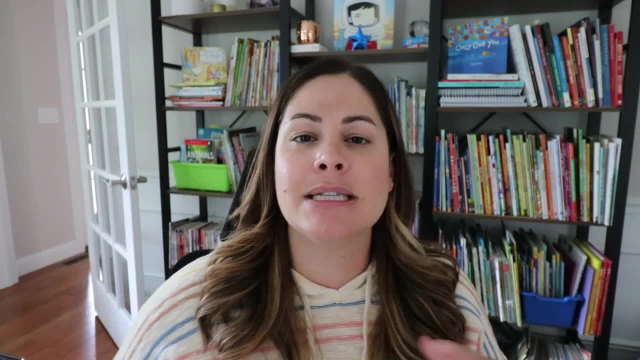 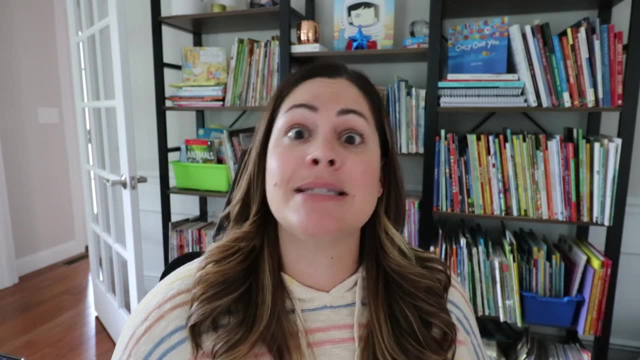 and that process of unitizing, As well as three different hands-on and more concrete examples and activities for you to use in your classroom right away. I really hope you're enjoying this series. My goal in each video is to give you lessons and activities that you can take and actually